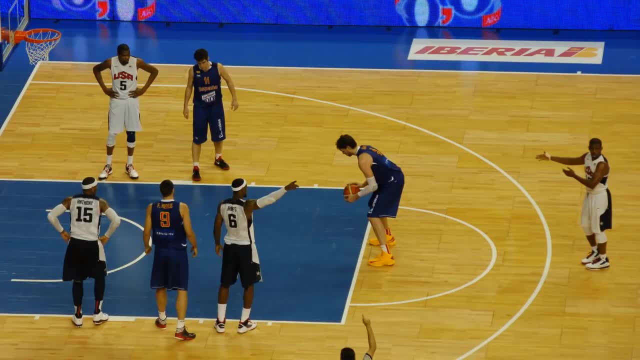 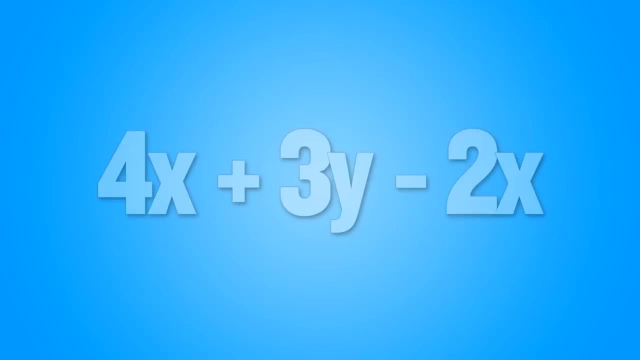 well with combining like terms is basically the same thing. we're looking for people or terms that have the same Jersey or they look the same. let's take a look at an alpha one example. we have the example 4x plus 3y and we want to use the same color, to have the same color as their teammates. 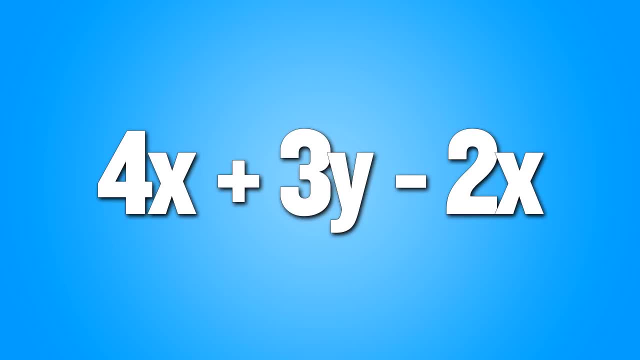 minus 2x. And if I were to ask you who is on the same team, who would you say: Yeah, that's right, 4x and minus 2x would be on the same team because they have the same letter or the same jersey. 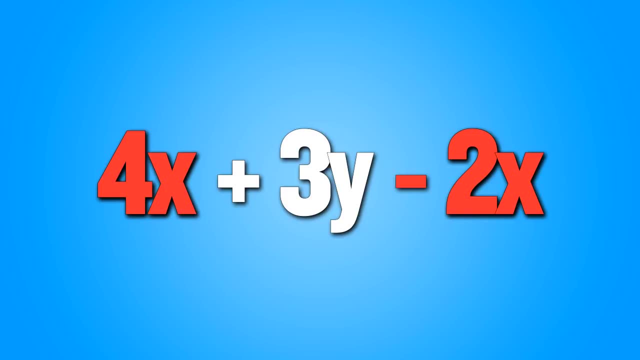 whatever you want to call it, they look the same. We're going to combine those, And here's the tricky part. When you're combining like terms, all you're worrying about is the big number in front. It's called a coefficient. Here the coefficients are 4 and minus 2, or negative 2.. We're only going. 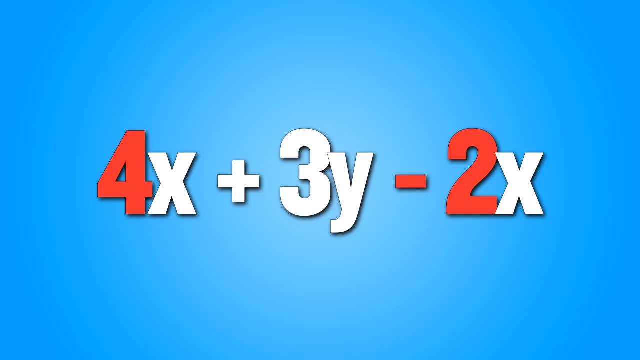 to combine those numbers. We don't worry about the letters, That's just the jersey. You don't need to do anything with it. right now We're going to do 4 minus 2, because there's that minus in front, which is 2.. And then you leave the jersey on because you don't want them to play without a. 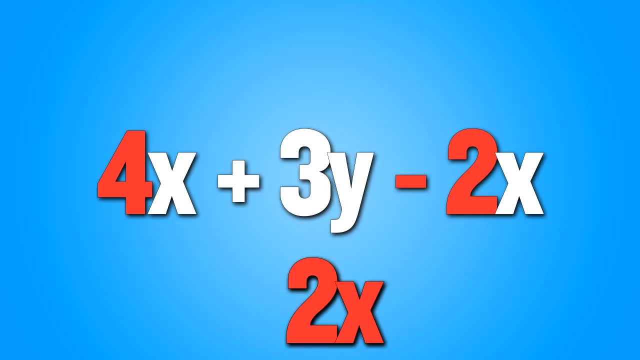 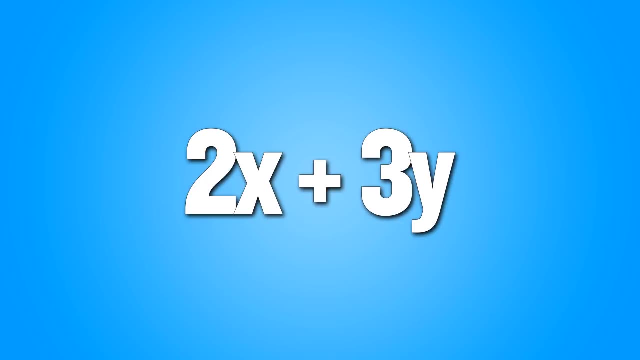 shirt: 4 minus 2 is 2, which will leave you with 2x, And we're left with 2x plus 3y. And our final check is to see if there's any more teammates after we simplify. Are there any more? No, because. 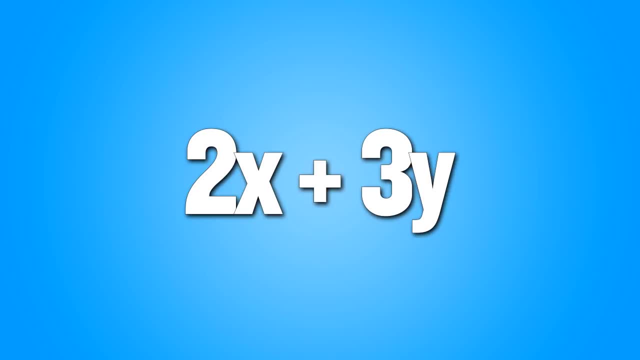 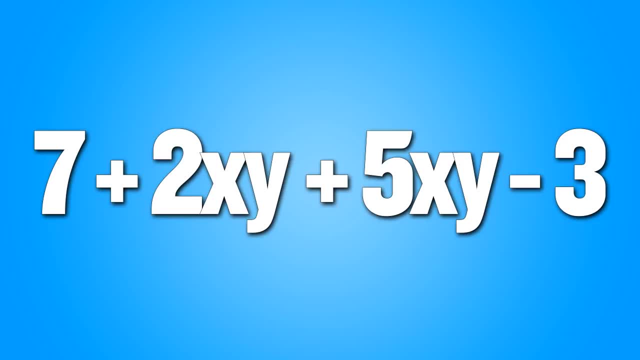 3. Once again, who's on the same team? Right away, I see that 2xy and 5xy look exactly the same. They have the same jersey, the same letters. Those are teammates. We're going to add those up because 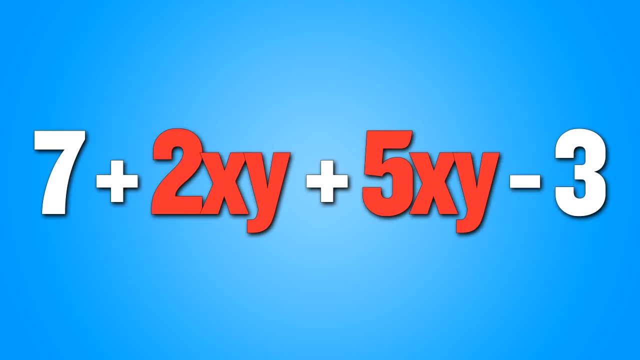 there's a plus sign in the middle: 2 plus 5 is 7.. We have 7xy. Let's go ahead and rewrite this. We got 7 plus 7xy minus 3.. And now we're going to add those up because there's a plus sign in the middle. 2 plus 5 is 7.. We have 7xy. Well, let's go ahead and rewrite this. We got 7 plus 7xy minus 3.. And we're going to add those up because there's a plus sign in the middle: 2 plus 7xy minus 3.. Looks like.